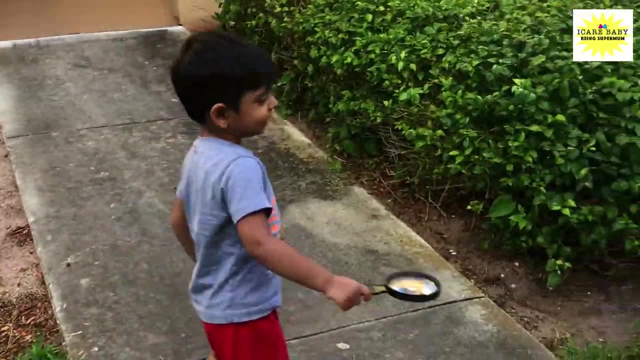 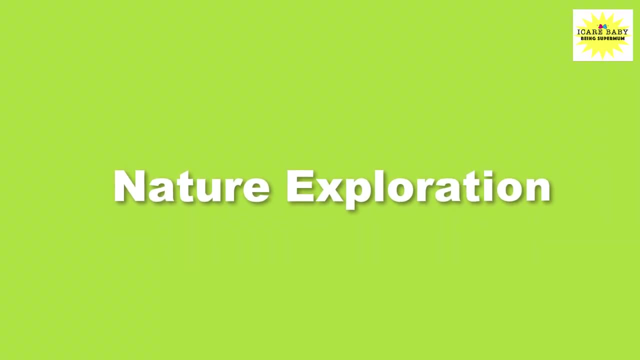 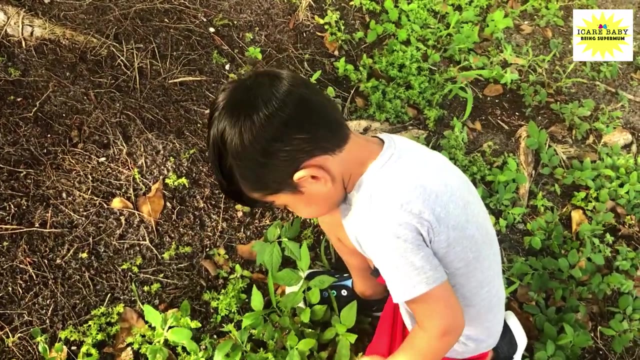 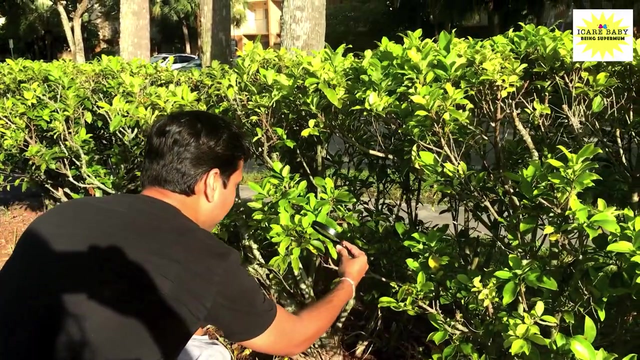 Hi mums and cutely babies. Welcome to- I get baby. Let's check out the nature inspired activities for toddlers. Nature exploration: A good way to introduce toddlers to nature, So let them explore the beautiful things that nature has to offer to them. So just take out your magnifying glass and go on a nature walk along with your toddler. 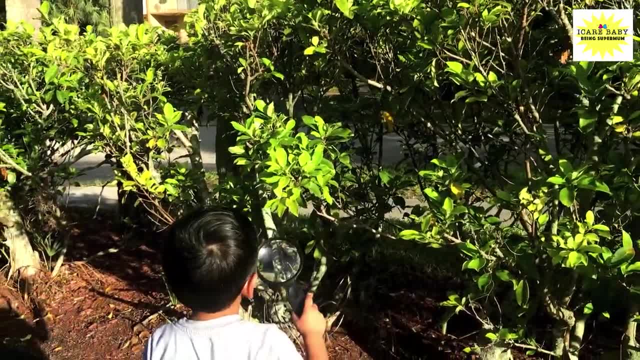 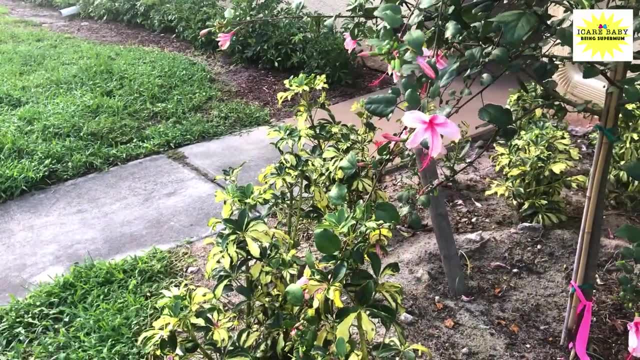 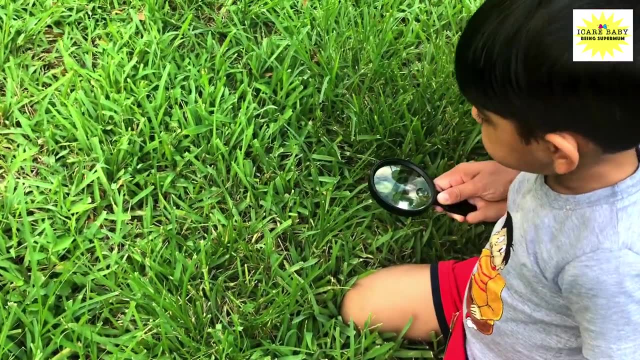 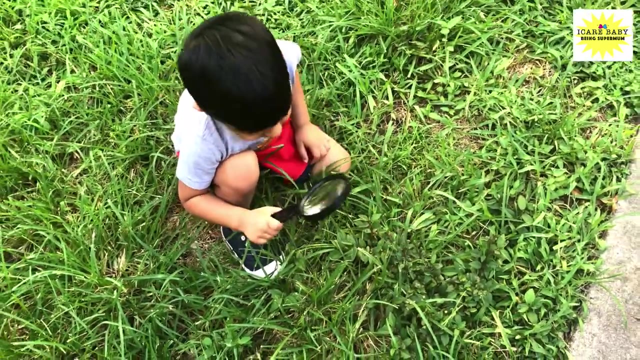 Exploring the nature is a good way of learning new things- words such as knowing about the different trees, plants, flowers, bugs, birds, etc. So encourage them for a nature walk and boost their curiosity by sharing the information about the things around them, As this can be a great way to spend some quality time with them. 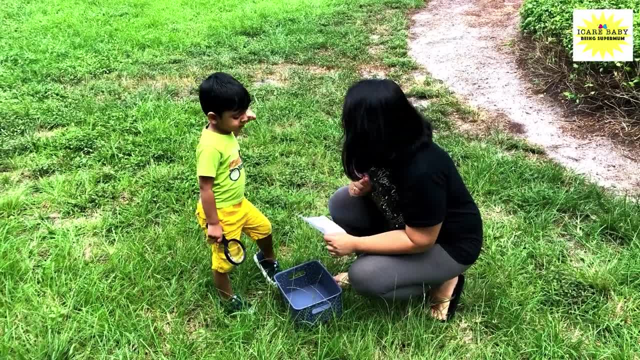 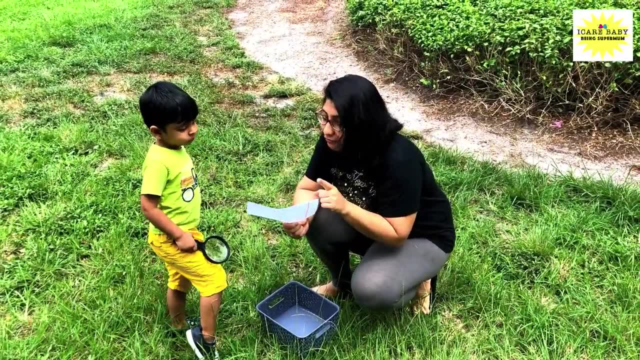 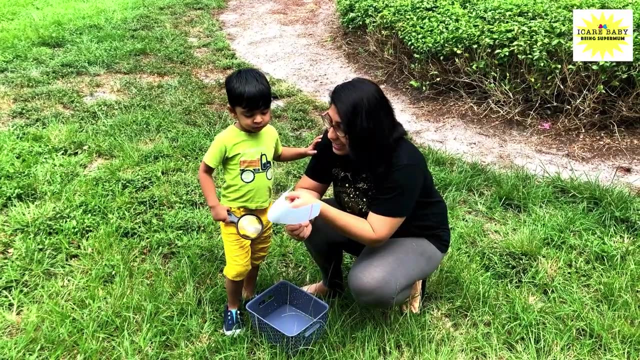 Okay, so today we are going on nature hunt- Yes, nature exploration. So we have to find out the things which is written on this page. We have to find first tree leaves, flowers, birds, grass, water, spider web, rocks, woodstick and sand. So are you excited to do this activity with me? 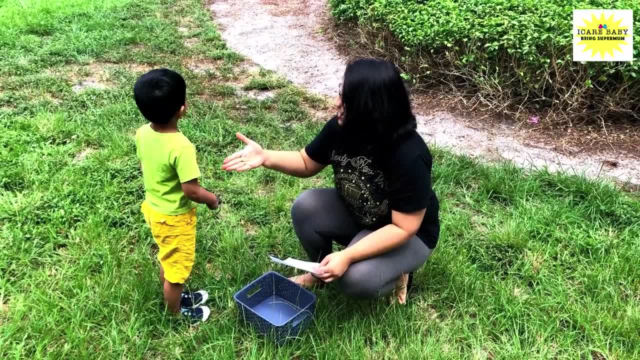 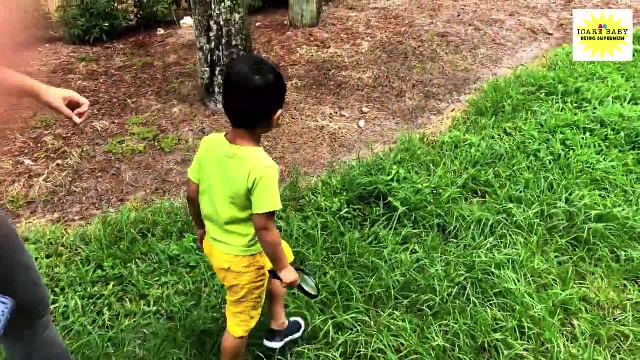 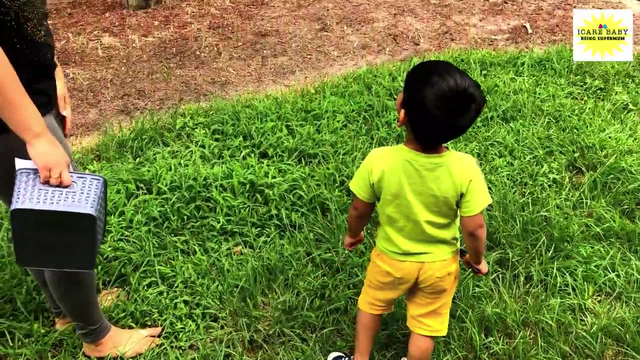 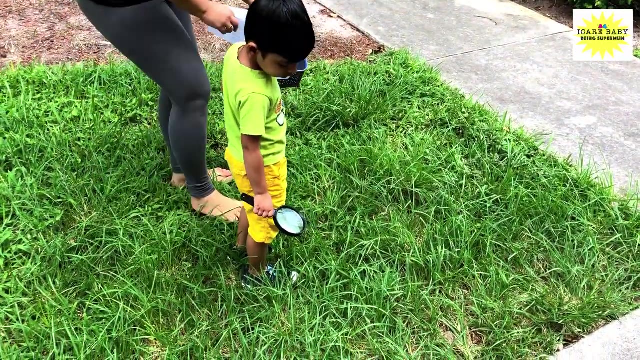 Yes, Can we do it? Yes, we can, We can Deal. Yes, Okay, good job, Let's go. Where is tree? Big tree, Big tree, yeah, Yes, where is grass Grass? Yes, can we pull some Grass leaves? I can't. 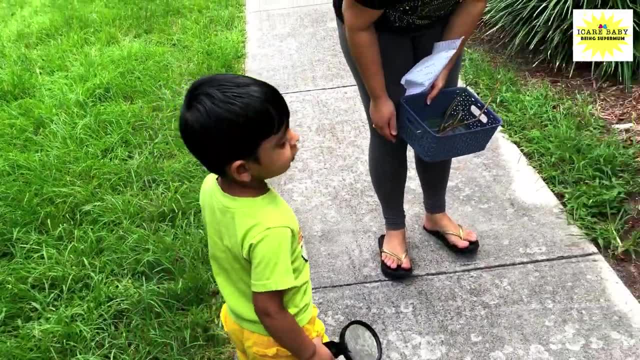 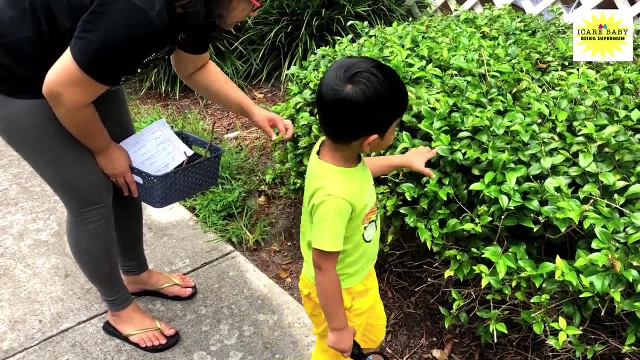 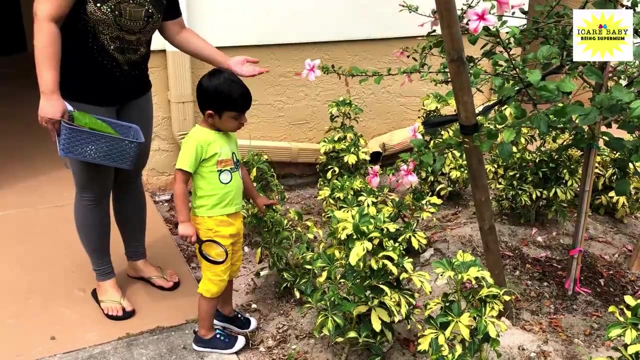 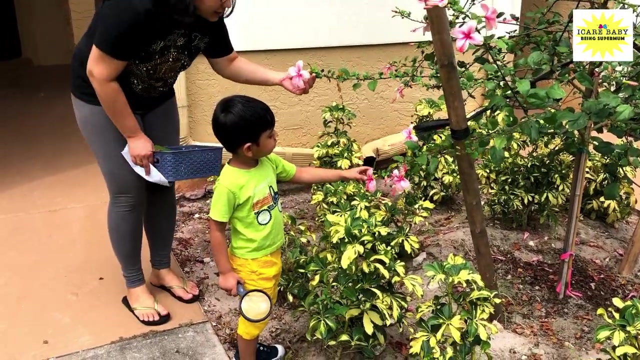 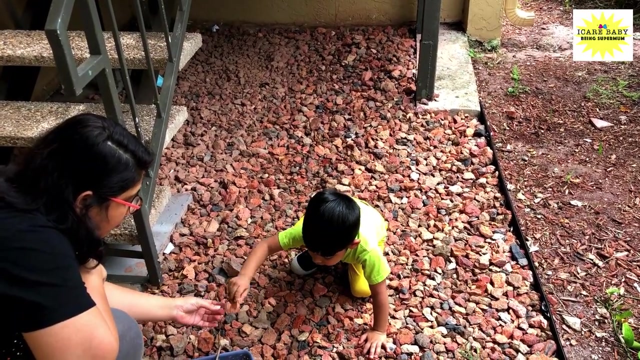 Yes, Where are leaves Leaf? Oh, it's a leaf. okay, So we'll just pick it up few leaves. Yes, Flower Flower is here. Yes, it's a dry flower. Wow, look at the beautiful colour. Which colour is this? Pink? Wow, good job. Only one, okay, Two.